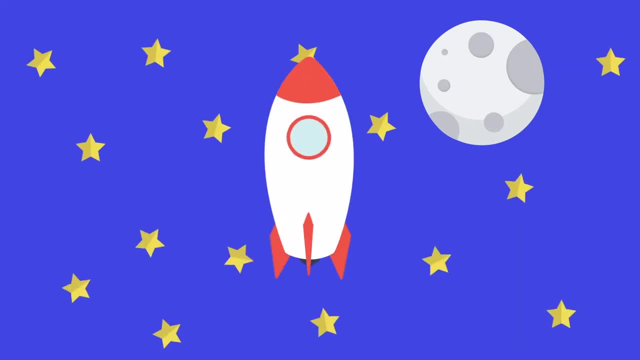 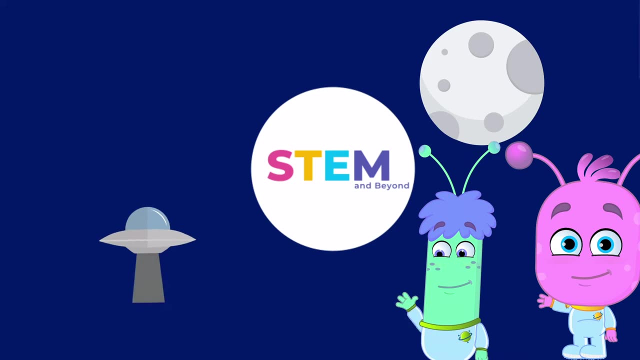 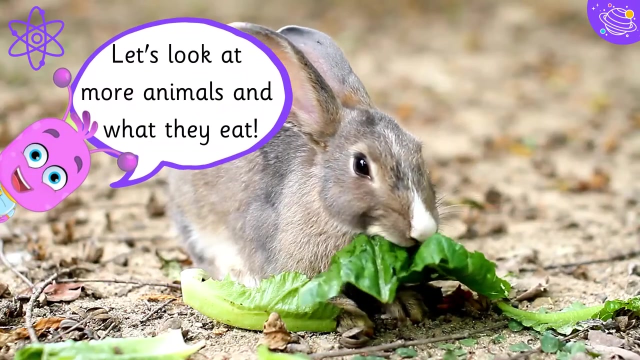 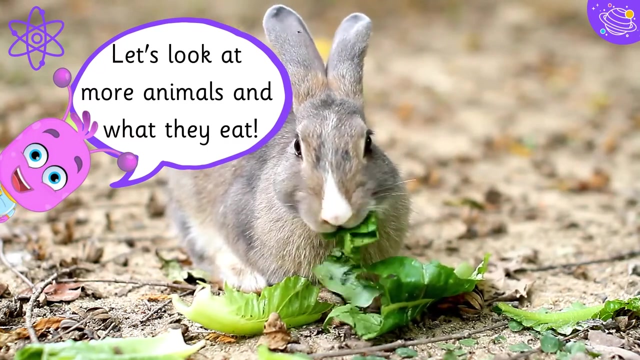 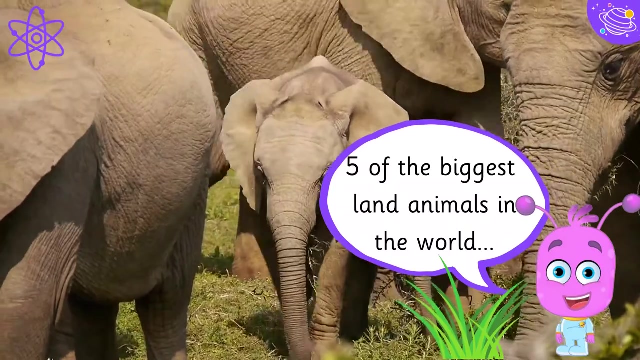 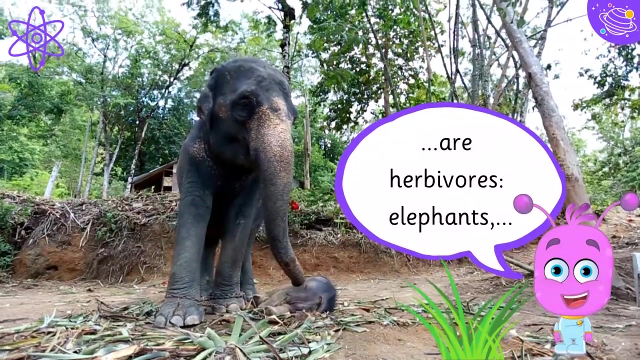 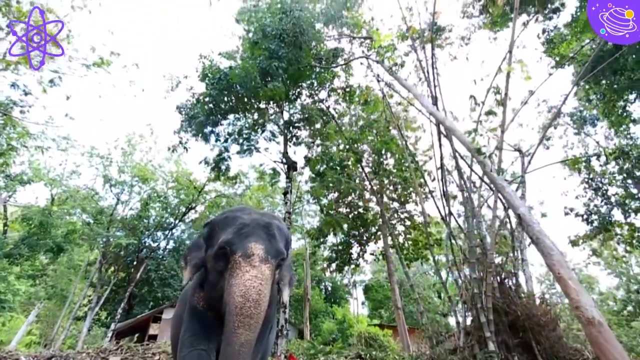 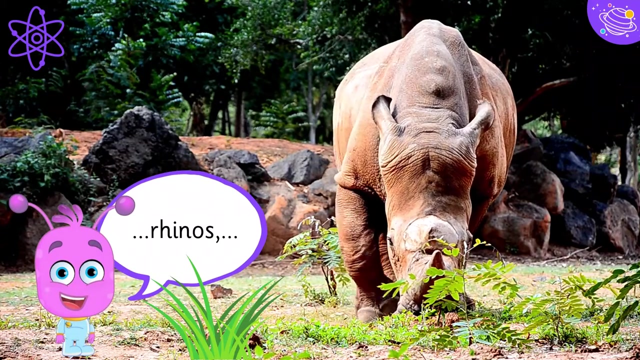 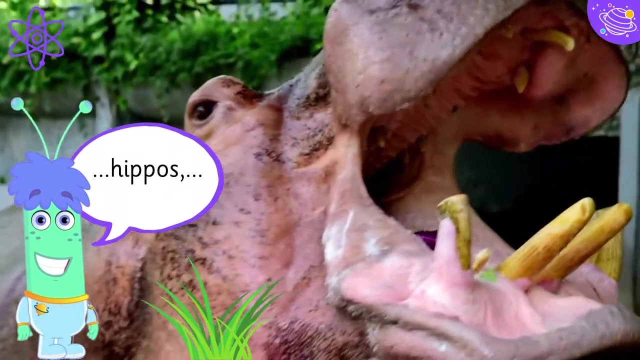 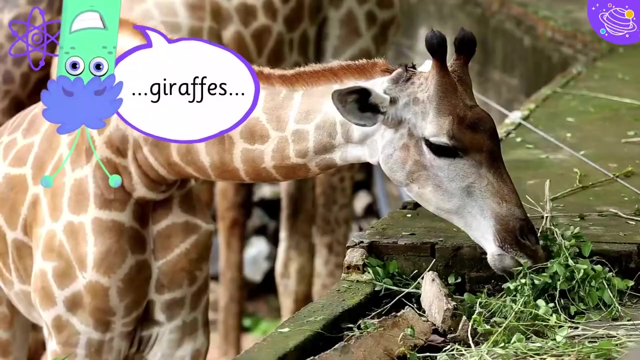 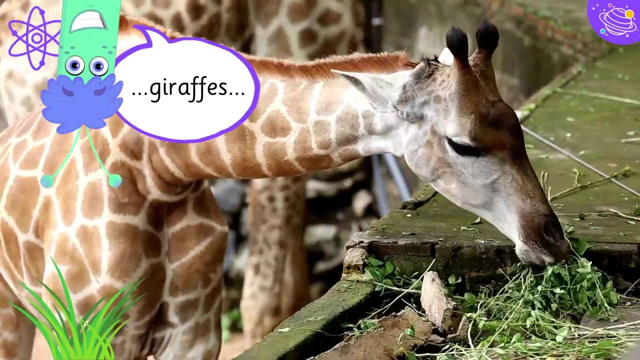 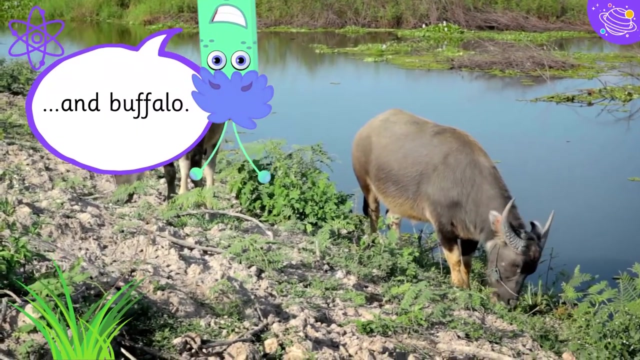 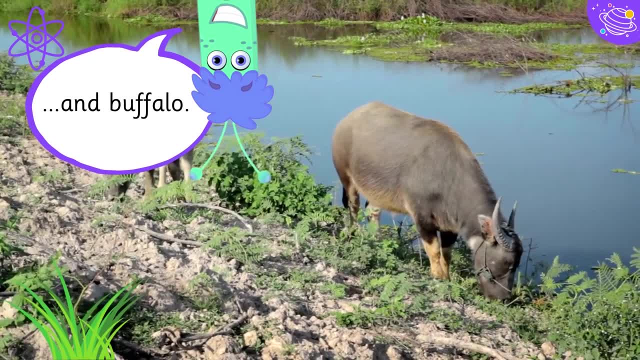 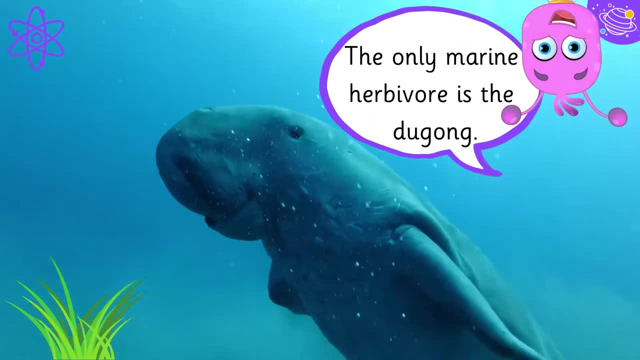 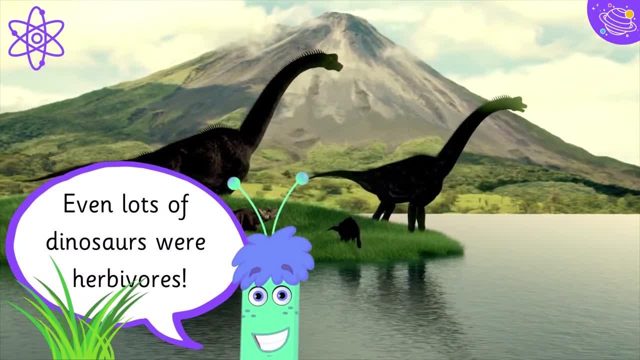 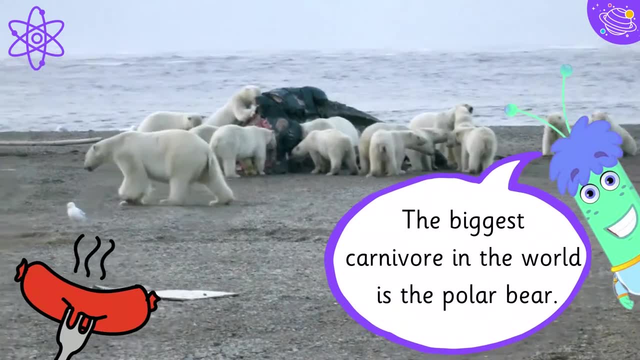 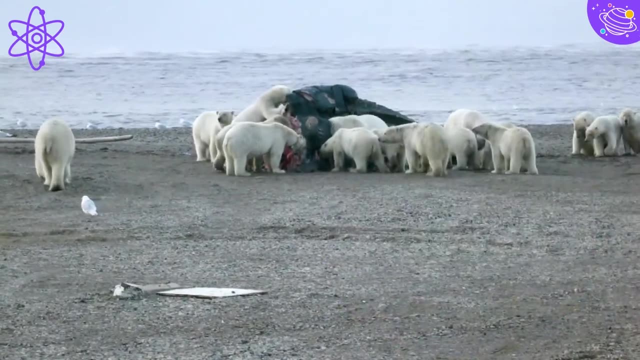 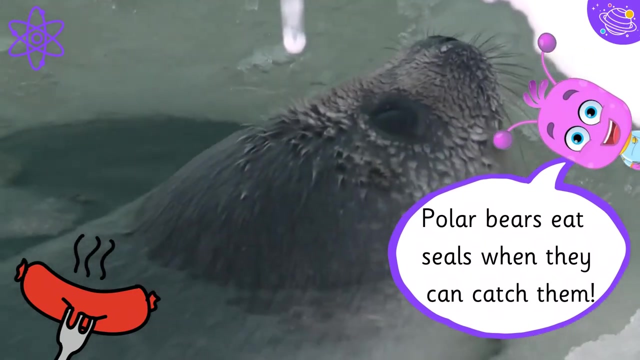 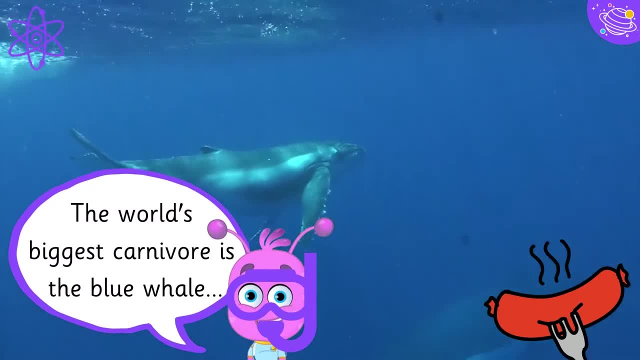 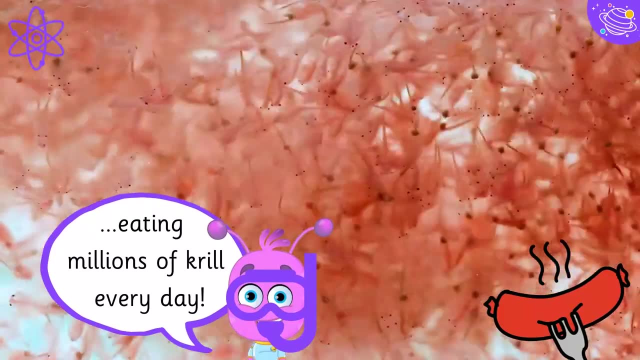 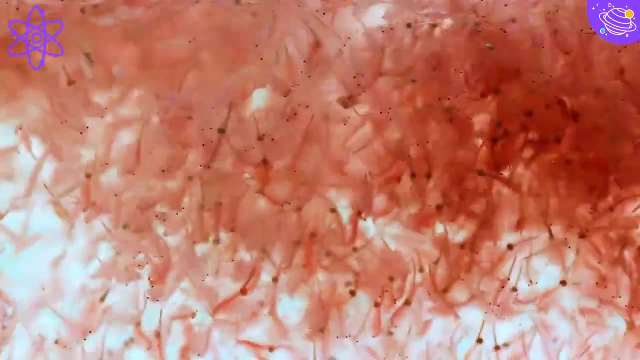 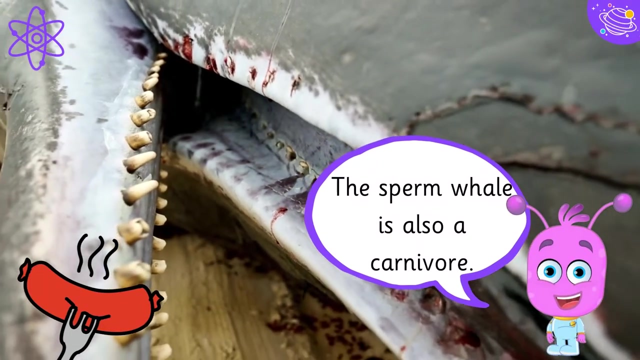 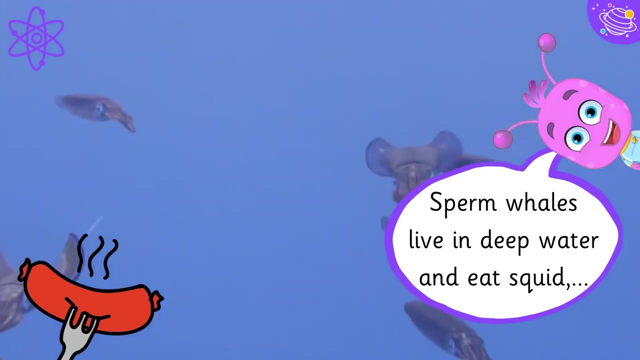 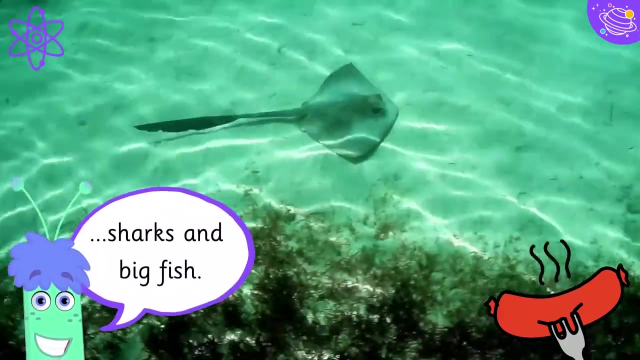 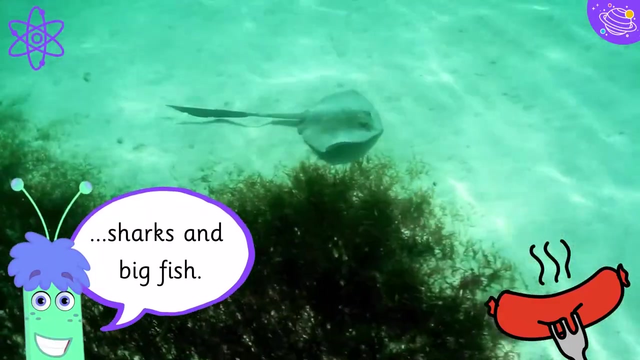 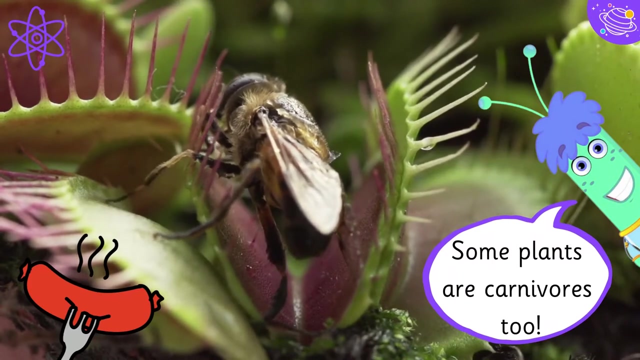 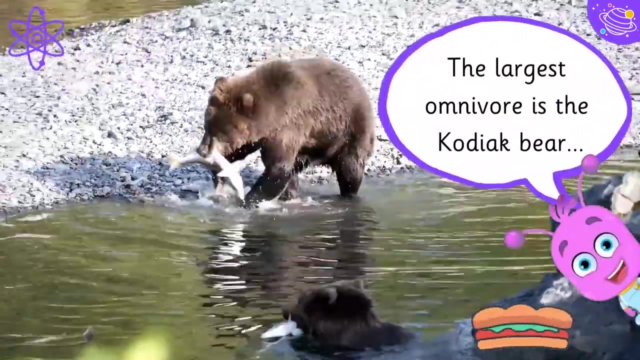 biggest carnivore is the blue whale, eating millions of krill every day. the sperm whale is also a carnivore. sperm whales live in deep water and eat squid, sharks and big fish. some plants are carnivores too. the largest omnivore is the Kodiak bear. 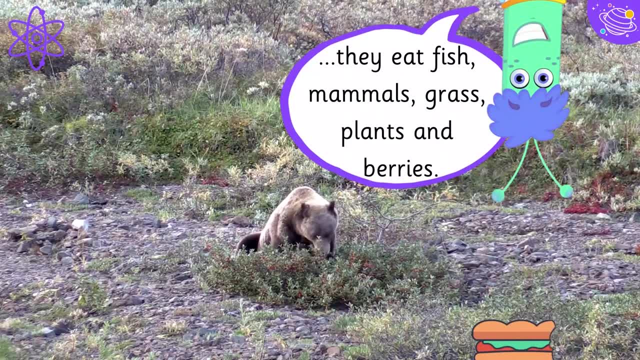 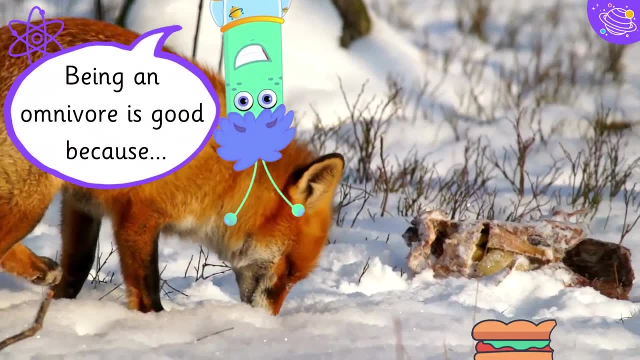 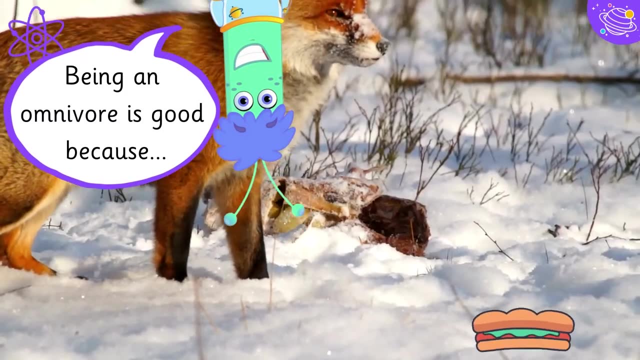 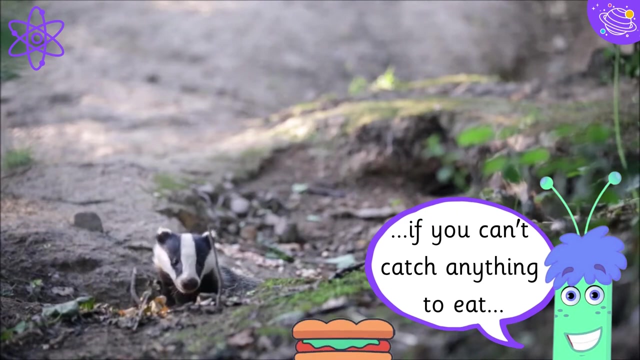 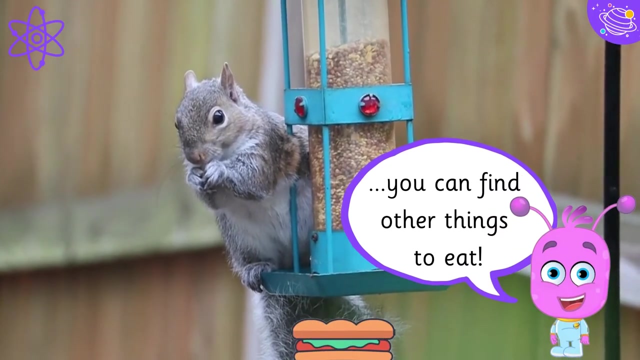 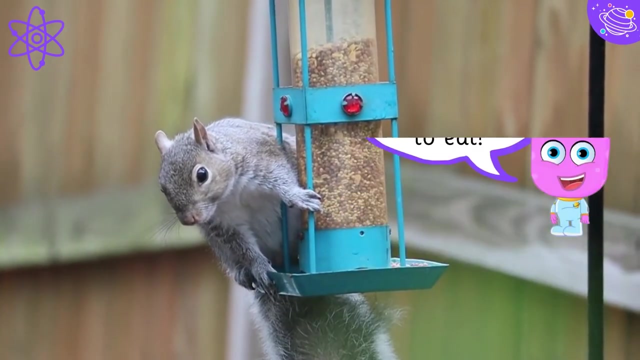 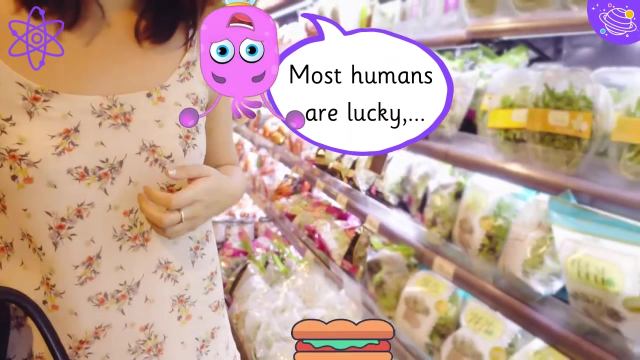 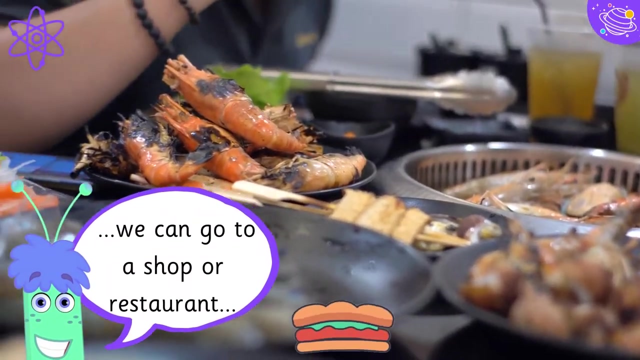 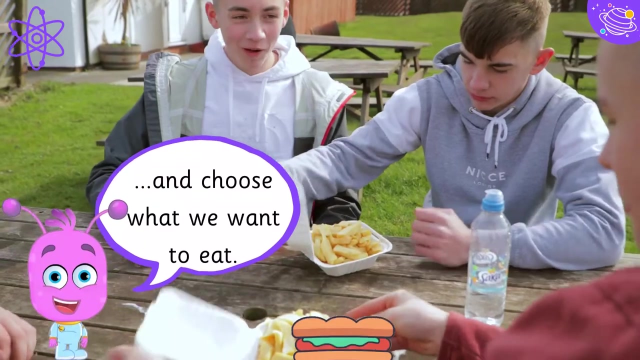 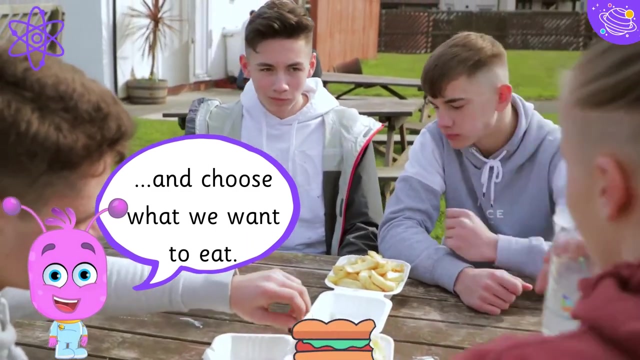 they eat fish, mammals, grass plants and berries. being an omnivore is good, because if you can't catch anything to eat, you can always find other things to eat. most humans are lucky. We can go to a shop or restaurant And choose what we want to eat. 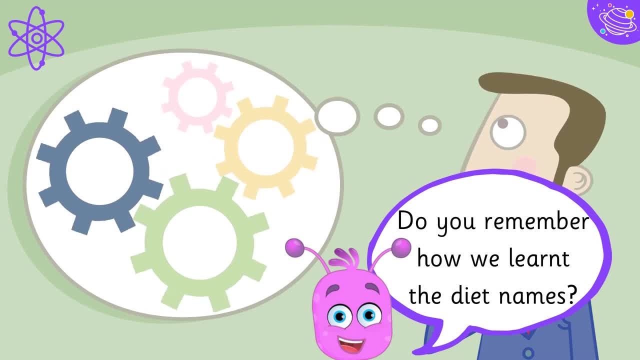 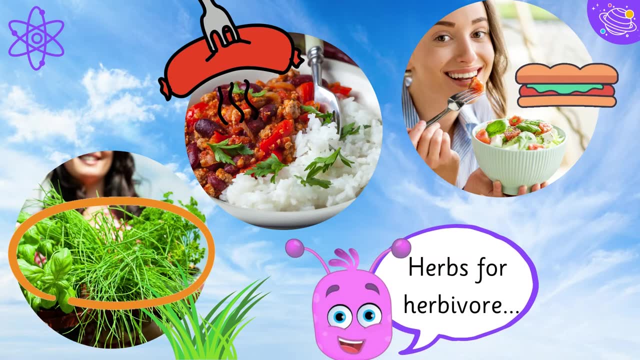 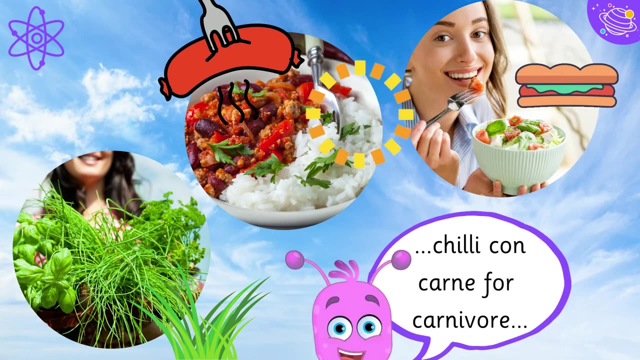 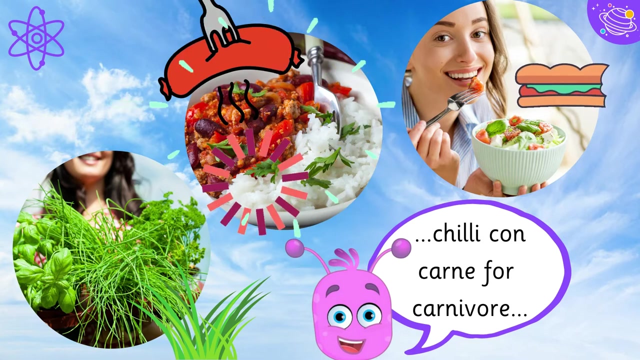 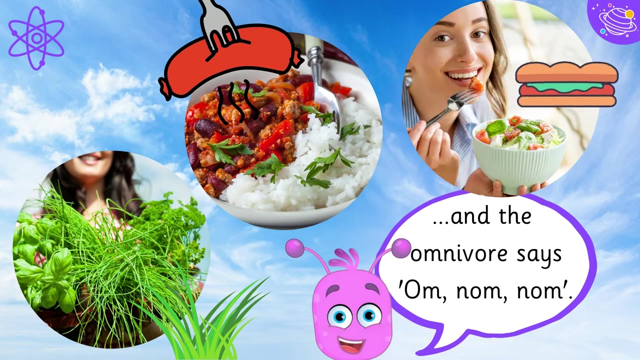 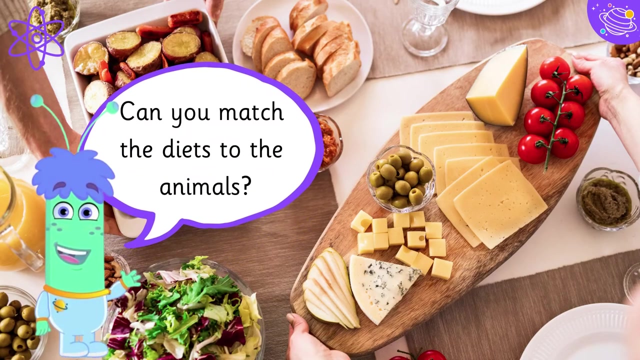 Do you remember how we learnt the diet names? Herbs for herbivore, Chilli con carne for carnivore, And the odd thing about carnivore is that it's called carnivore for carnivore. Omnivore says om nom, nom. Can you match the diets to the animals?